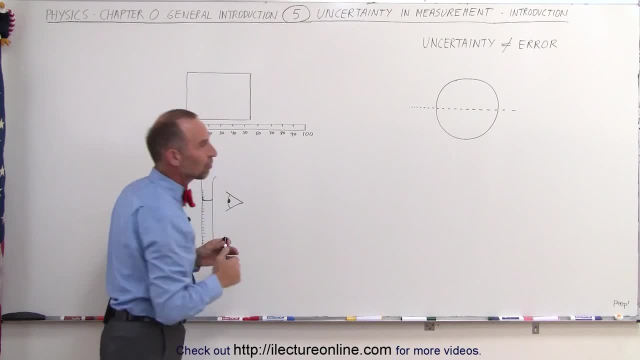 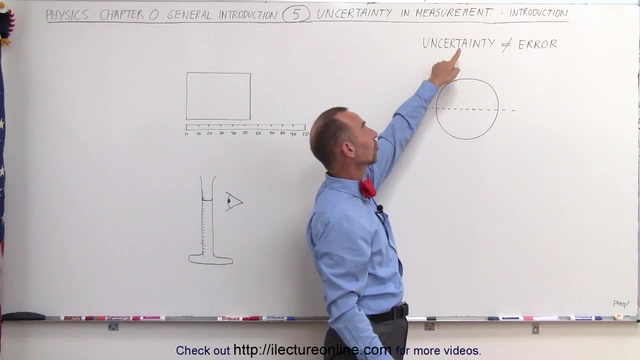 eyeball it. you try to figure out. well, where is that exact measurement? what's the best you can do? Notice we're not talking about an error in the measurement. Notice what I have up here. uncertainty is not the same as error. When you make an error, you simply make a mistake. You thought you read 50, but 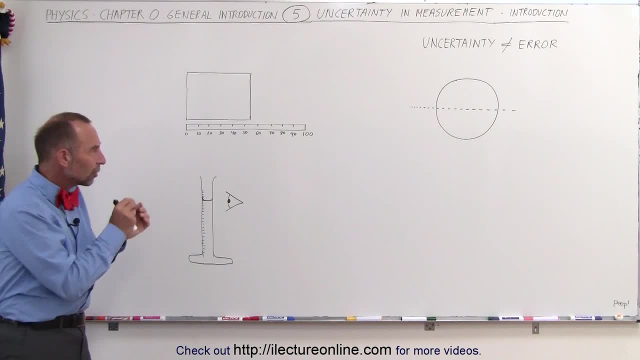 it was actually 60.. That's an error, that's not an uncertainty. But when you sit there and you say, is it 54 centimeters? is it 55 centimeters, is it 56, I can't really tell because my eyesight isn't very good or the lighting conditions are. 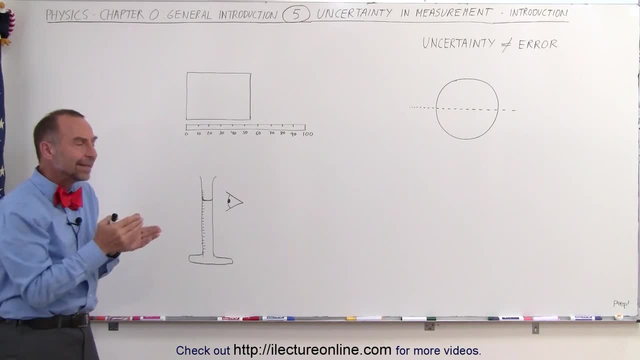 bad or the ruler doesn't have very good markings or so forth, then you have a certain amount of uncertainty in the measurement and you have to account for that. when you take the actual measurement, You have to write down what you think the uncertainty is. Now, uncertainty is sometimes very poorly. 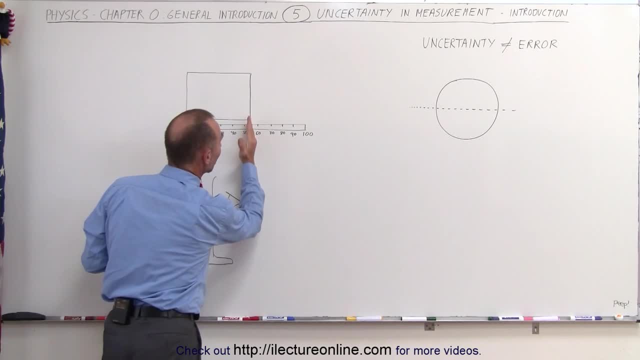 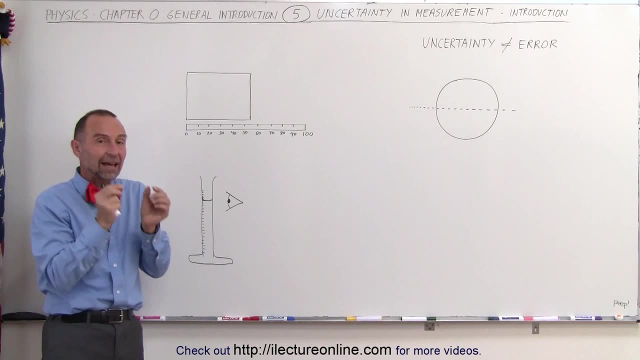 understood. Most of the time, people will look at this number right here and think, okay, whatever the smallest graduation is, let's have a meter stick, and the meter stick has graduations down to the nearest millimeter, whatever the smallest graduation is on the scale. they will then say: well, the uncertainty is plus, or? 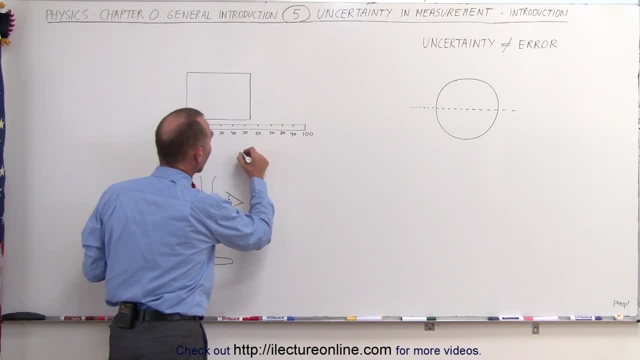 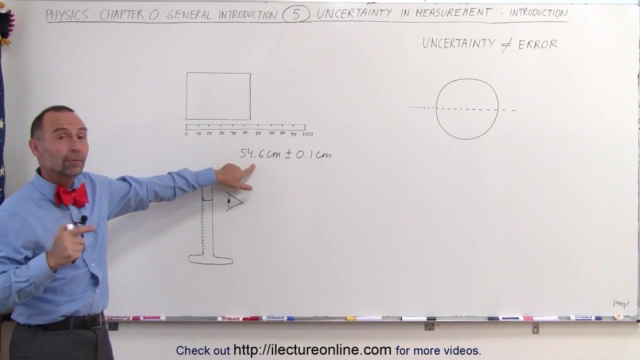 minus that smallest graduation, For example, they will write down: well, it looks like it's fifty four point six centimeters plus or minus zero point one centimeter, because that's the smallest graduation on the meter stick. But there's a lot of other reasons why you may not be very certain about the 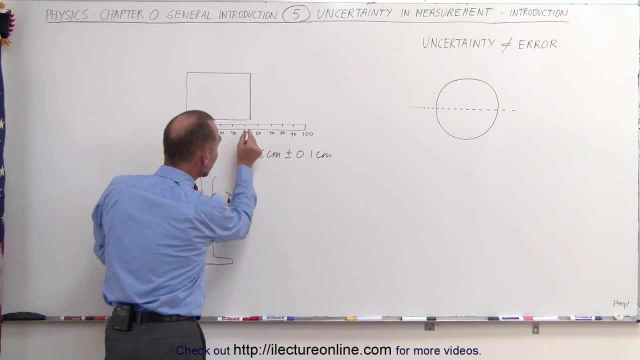 accuracy of this number. For example, how do you know that you're looking at it at the right angle? When you have a slight deviation from the angle that you look at, the number here can easily change to fifty four point eight, or fifty four point four, or fifty four point two, depending upon how you look at it. The 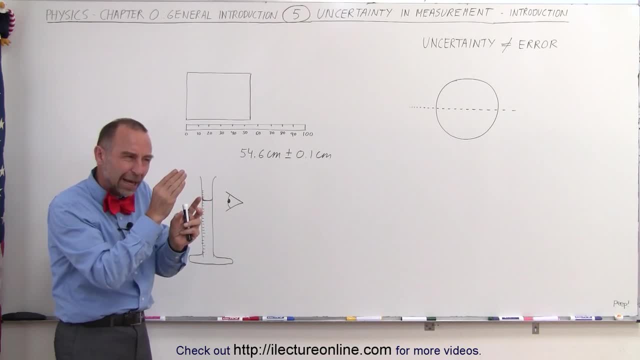 lighting conditions could be pretty bad and therefore you can look at it and you can't really tell that carefully. There may be some shadows there that make it hard to see. It could be that your eyesight isn't that good and therefore you're not quite sure what the line is. Is that the third line? 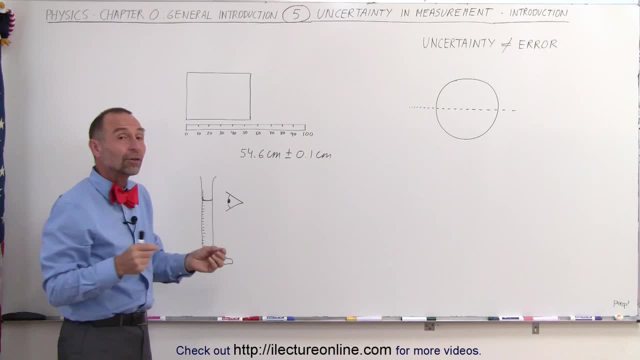 the fourth line. You can't really tell. Sometimes it's simply a matter of you don't have a lot of experience at using the tool. Now, a meter stick is a simple tool that most people know how to use, but there could be all kinds of other. 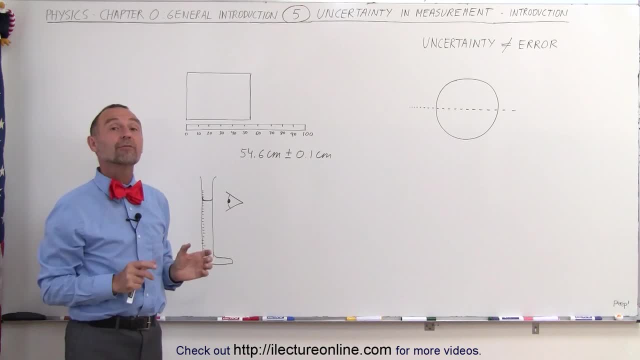 apparatus that you must be using and you may not be very familiar with it, and so you're not quite sure how to do it quite correctly. Also, what people ignore is- you may have an uncertainty here- and exactly lining up the end of the of the ruler with the end of the object, There could be a certain amount of. 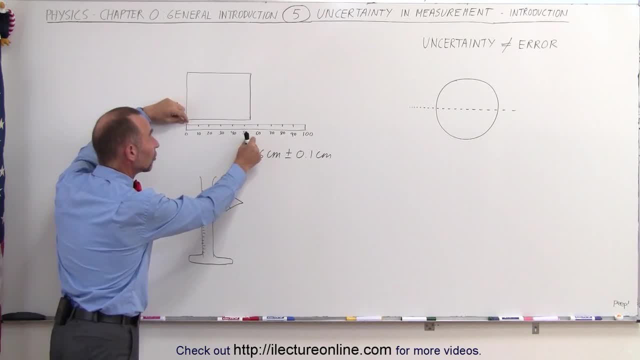 uncertainty here as well, and you have to add this uncertainty with that uncertainty and all the other factors that come into play. So it could be, under the correct circumstances, that the best you can do is maybe to the nearest half a centimeter, and so, therefore, what you would write is: you say: well, it's fifty. 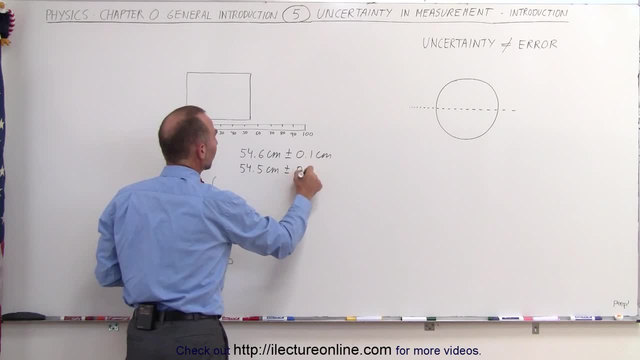 four point five centimeters plus or minus zero point five centimeters. If the uncertainty is 0.5 centimeters, you definitely don't want to go too accurate here on that, That last decimal place here, and on the decimal place past the centimeter, You 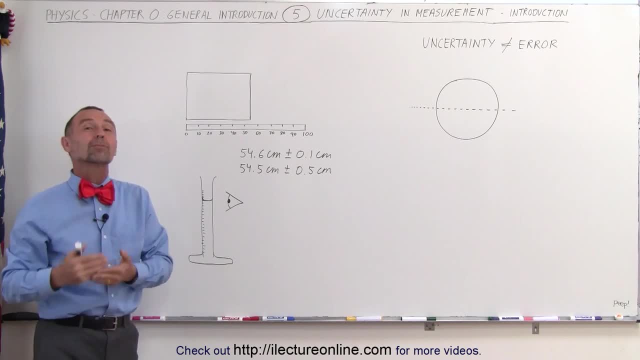 don't want to write: it's fifty four point four, nine centimeters plus or minus 0.5 centimeters. You want to kind of line it up a little bit. So what this is really telling you is that you're not quite sure if it's fifty four point five, could. 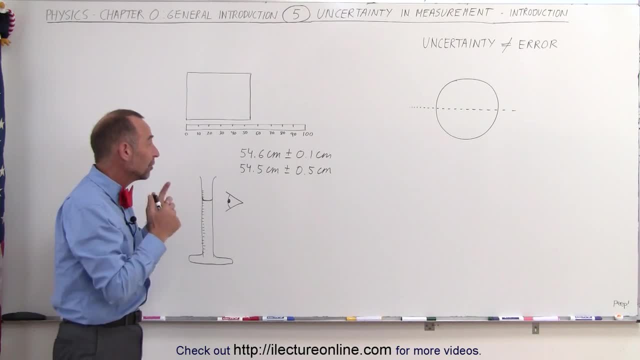 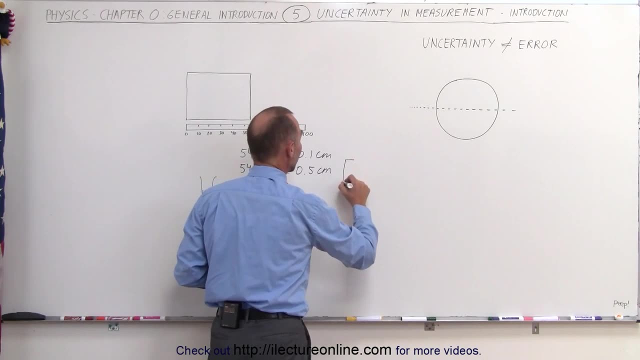 have been fifty four point eight, could be fifty four point two, but what I do know that it's not bigger than fifty five and it's not smaller than fifty four. This tells you that your measurement is somewhere between fifty four point zero centimeters and fifty four point five. 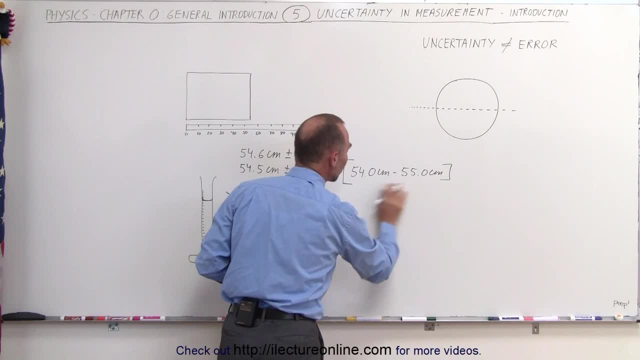 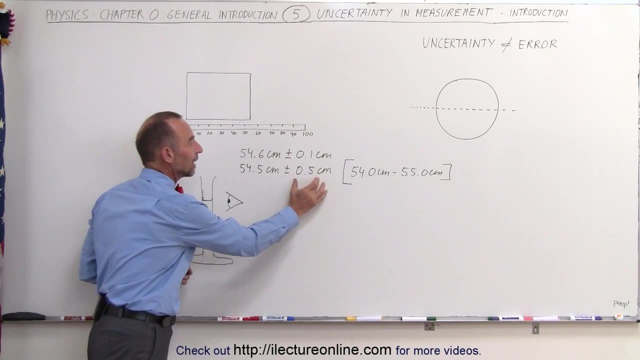 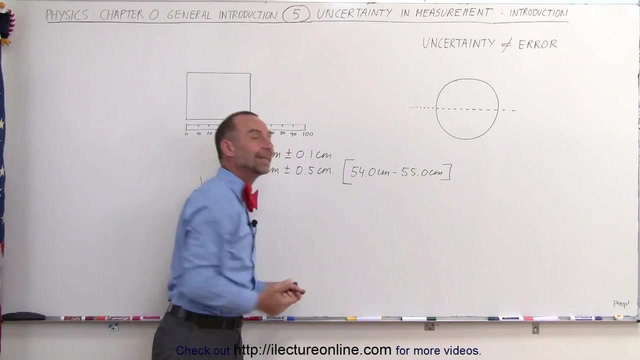 Fifty five point zero centimeters. It's really somewhere between those two. I am almost a hundred percent sure that the measurement is somewhere between here and that's indicated by this. So that you add this to this, it gives you fifty five. subtract from this gives you fifty four. You know that the range here 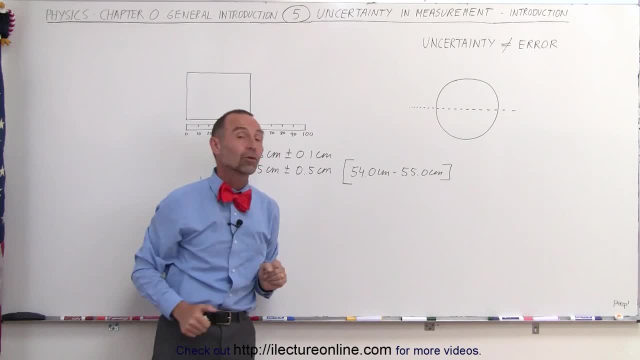 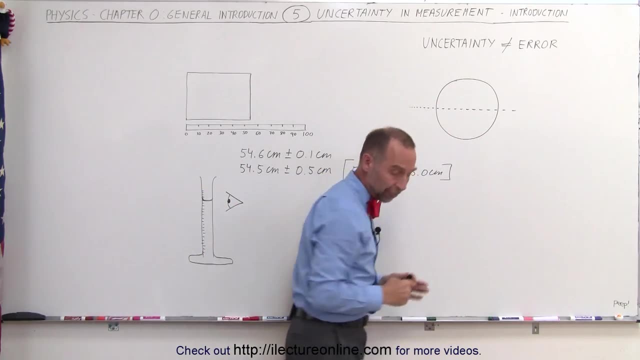 indicates. that is the certainty that you have. that is somewhere between those two values. Now, other reasons why you may have uncertainty: Let's say you're trying to measure the diameter of a particular circle. Let's say you're trying to measure the diameter of a particular circle. 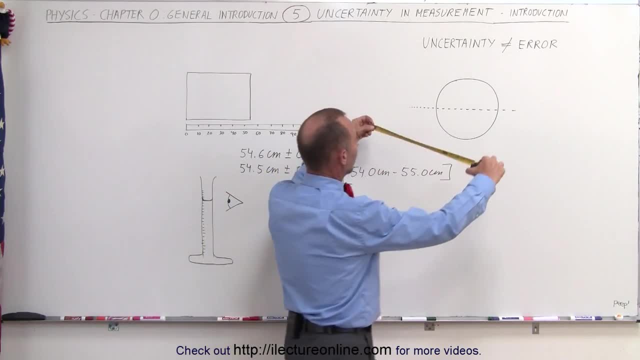 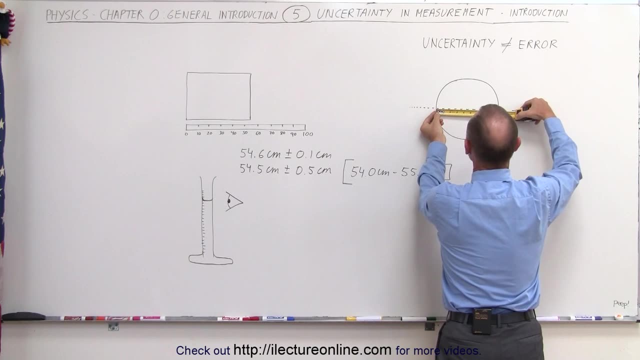 And so if you take a measuring apparatus like a ruler, like this, So first of all you have uncertainty where exactly you're going to line it up at the edge, And then you're not quite sure if you're holding it just right. Are you measuring? 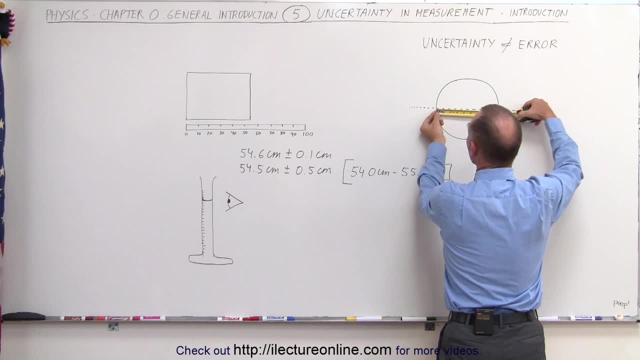 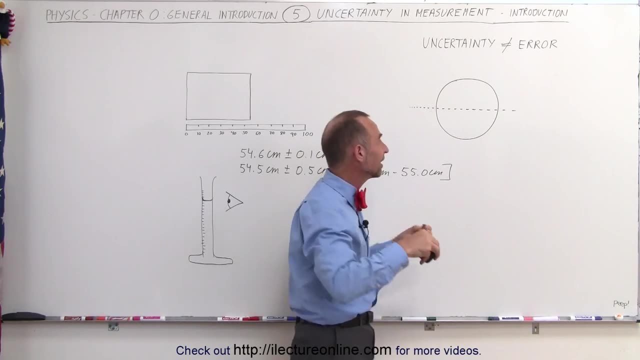 it at its widest as a diameter, or you're actually cutting the line a little bit so that you're actually measuring something that's smaller than it actually is. It may be difficult to figure out where exactly the diameter of the circle is, So simply lining it up may be difficult. Or, for example, let's say: 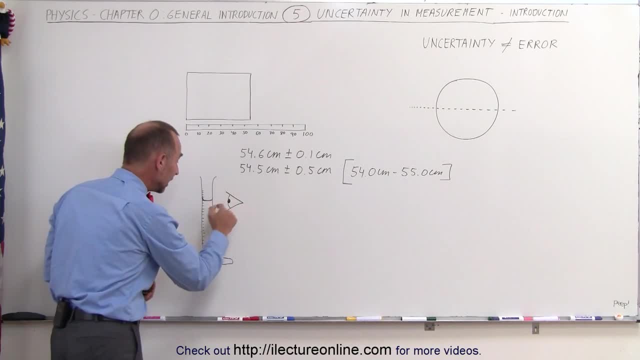 a liquid inside a graduated cylinder. Again, you may be looking. You're looking at there's a meniscus at the very end. You're trying to find out, line up where that bottom is. You're trying to line that just perfectly. You could be off You. 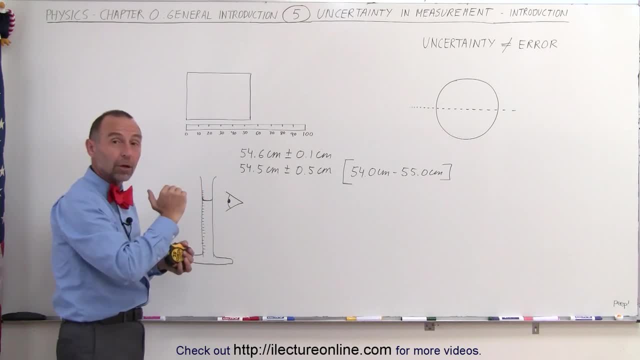 could be a little bit above, A little bit below the line And as you're being above or below the line, you may be looking at the wrong marking right there. Again, you may look at it and say: well, in milliliters, the amount of the 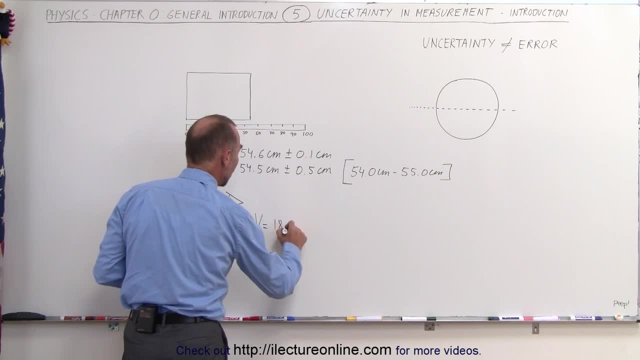 volume in there. So you say the volume is equal to, let's say, eighteen point two milliliters. So you say the volume is equal to, let's say, eighteen point two milliliters, But you're not quite sure. You could be one or two graduations above or below. 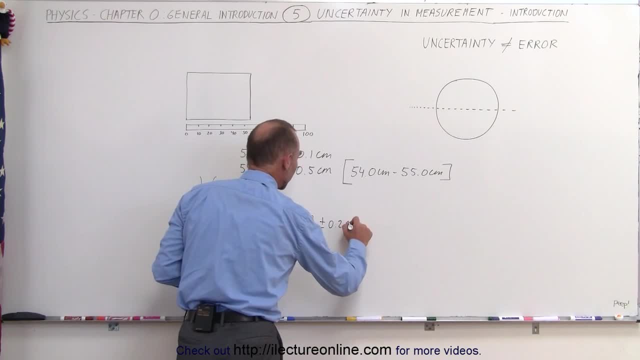 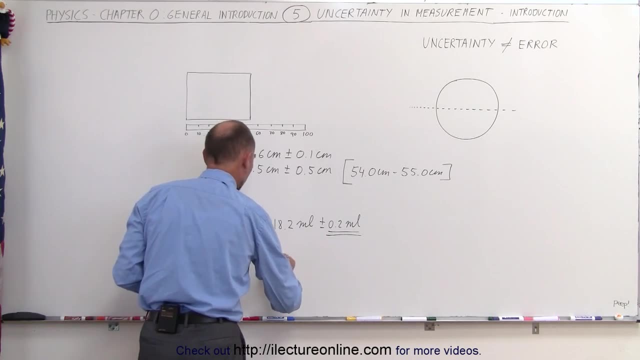 Then you say, well, that's going to be plus or minus 0.2 milliliters, And this then becomes the uncertainty. What you're telling everybody is, when you made that measurement, that the volume is somewhere between the value of eighteen point four milliliters and eighteen point zero milliliters, And that is the best you can. 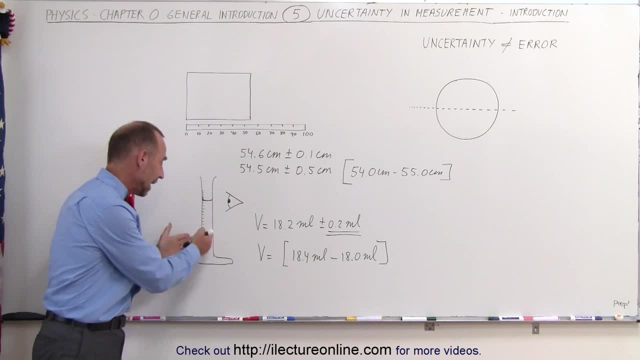 do. You cannot be any more accurate than that, given the quality of the apparatus, Your ability to read the scale, the lighting conditions, the shadows, the angles that you have and all the other uncertainties creeping into the measurement. You must indicate that it's somewhere between 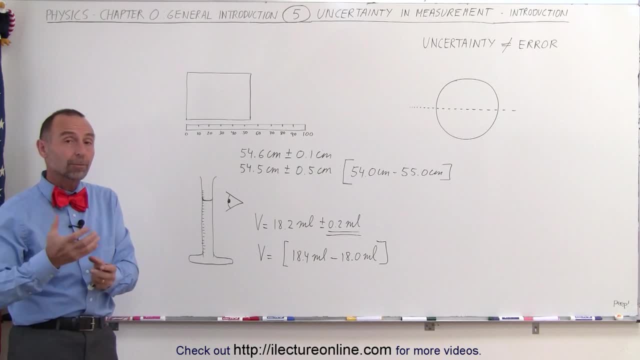 those values. So what do you do now when you have a number or a set of numbers that you measured, and now you're trying to find the volume, You're trying to find the area, You're trying to find the density of something, using values that have uncertainties in them. Well, 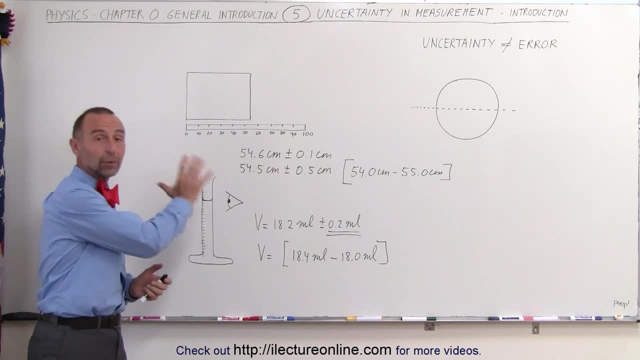 we need to learn how to deal with those as well. So, first of all, understand what uncertainties are- They're definitely not errors- And then, in the next video, we're going to show you how to actually use numbers that have uncertainties with them to actually calculate the final values. 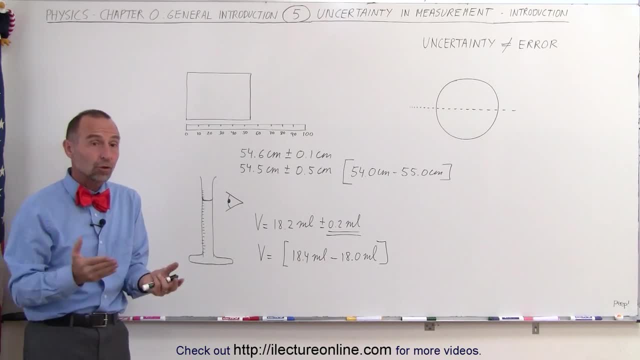 You always have to take into account that the numbers you're using are not absolute correct numbers. They have a certain amount of range in it where you're not quite certain what the correct value was, And that's how we deal with uncertainties.